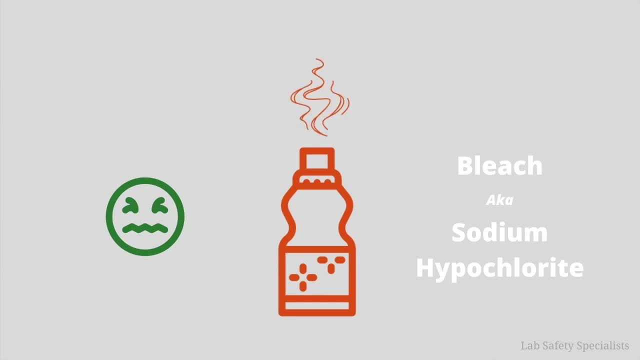 unstable in solution, which causes it to release chlorine, which is the active principle of the bleach. On its own, these bleach-based solutions are strong enough to remove stains and kill microbes and even corrode metals. As you might expect, this can do a bunch of damage to your body. 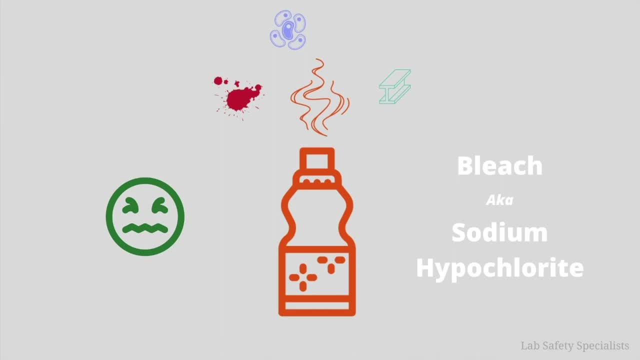 especially if it makes contact with mucous membranes or becomes ingested. That's just bleach on its own. Go on. Sodium hypochlorite is known for its reactability with other chemicals. The most infamous of these reactions is with the chemical ammonia. Ammonia is 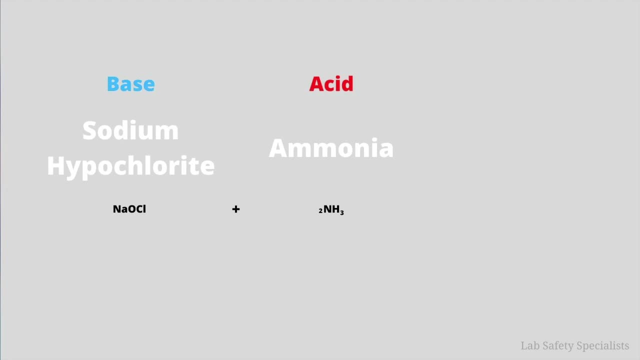 is an acid, while sodium hypochlorite is a fairly weak base. When the two meet, toxic chlorine gas is released, which has been used as a chemical warfare agent and can kill you at high enough doses, Even if these vapors don't kill you. 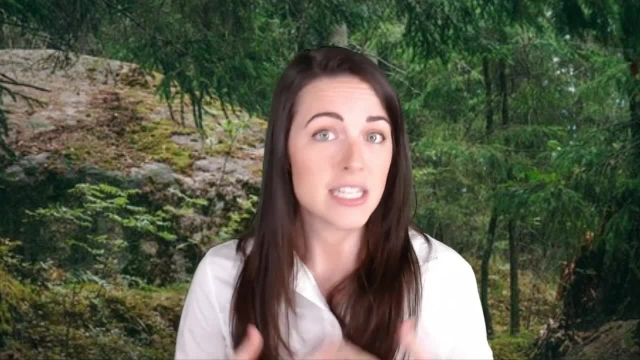 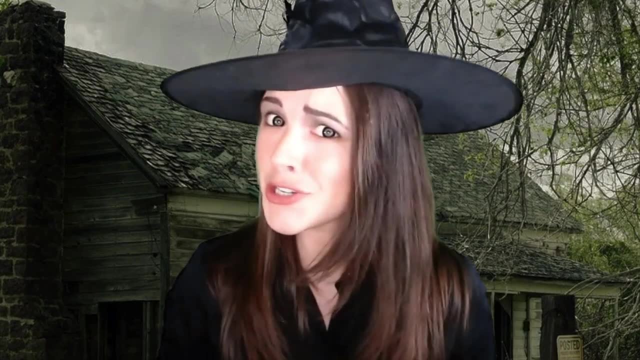 you probably won't like the side effects: Coughing, sneezing, shortness of breath, nausea, even pneumonia. Okay, but I'm fairly sure I've never bought anything called ammonia. All of this is just from my cottage. 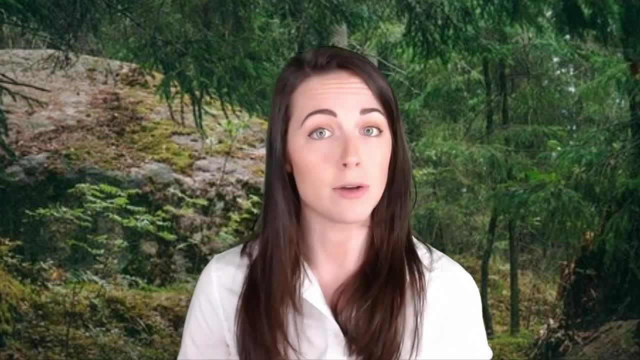 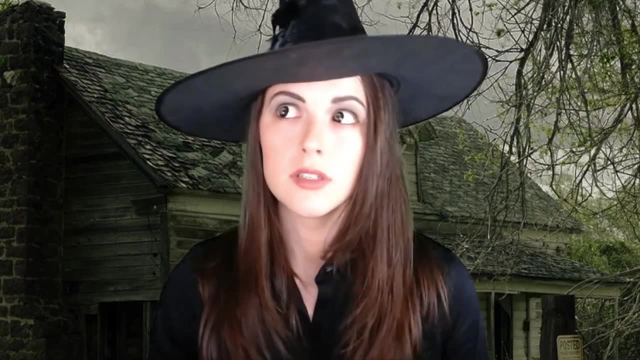 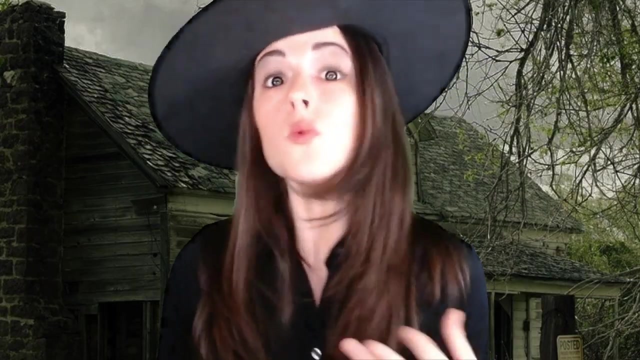 Like sodium hypochlorite, ammonia, can be found in a lot of household cleaners and products: Glass and window cleaners, interior exterior paints, Oh, and also urine, Okay, well, regardless, how would one stay safe? I am so glad you asked. 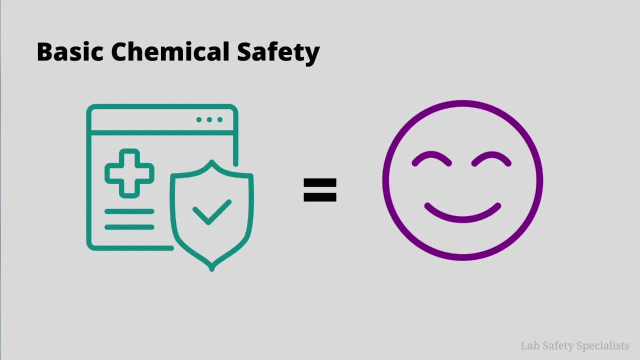 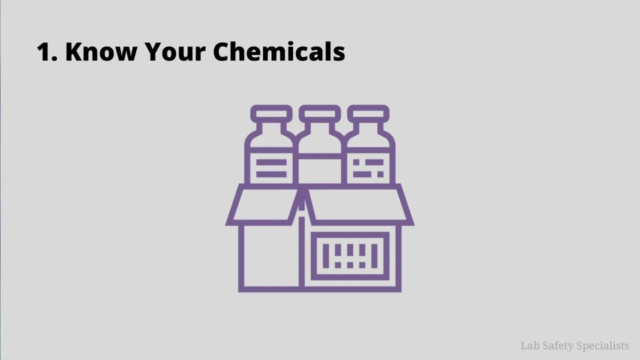 To stay safe while using dangerous chemicals, here are some basic rules. First, always know what chemicals you are dealing with. The easiest way to do this is to carefully label all of your containers as you fill them and make sure that everything has a list of potential hazards. 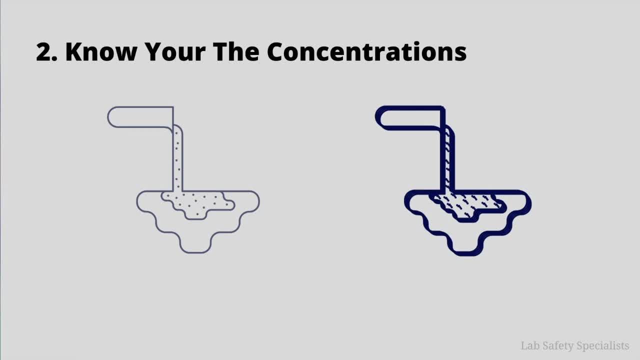 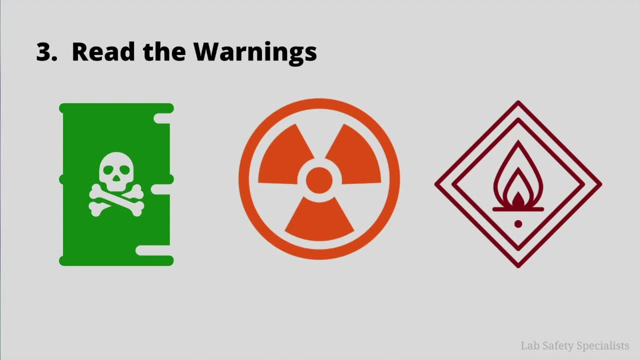 Number two: you need to know your concentration of your chemicals. Even household chemicals vary in their concentration. Read all the warnings about adverse reactions. These may be listed on the chemicals packaging. When in doubt, you can do a quick web search or check your laboratory's MSDS. 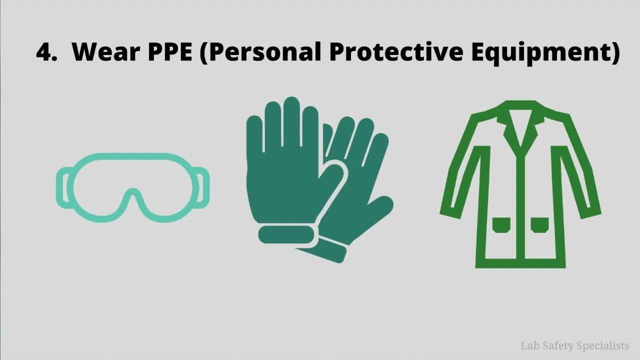 material safety data sheets for guidance. Speaking of precautions, always be sure to wear the proper personal protective equipment and work somewhere where any spills, fumes or unexpected accidents can be dealt with. Super, really scary. definitely fits the whole aesthetic.